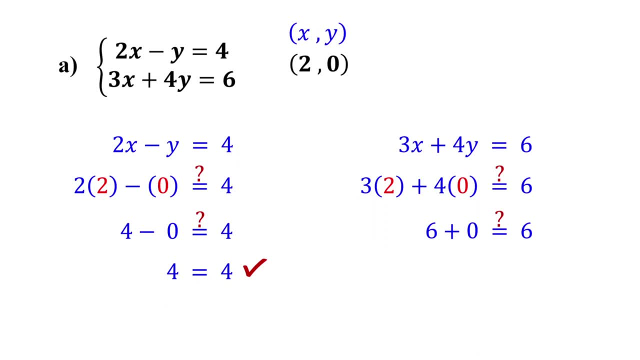 3 times 2 is 6 and 4 times 0 is 0.. 6 plus 0 is 6 and 6 is indeed equal to 6.. So it also satisfies the second equation. Therefore, since the ordered pair makes both equations true, it is a solution to this system of equations. 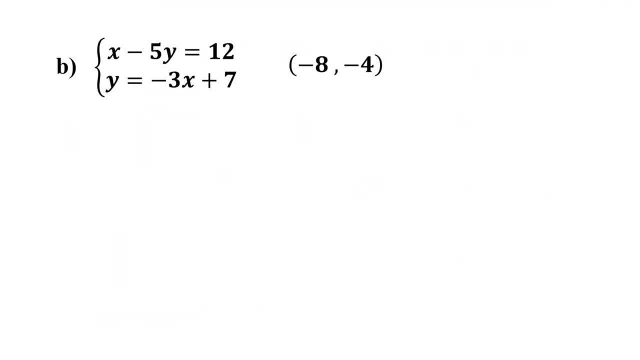 Now let's move on to the second example. Does the ordered pair satisfy this system of equations? Negative 8 is the x value and negative 4 is the y value. Just like before, our initial step is to substitute these values into both equations. 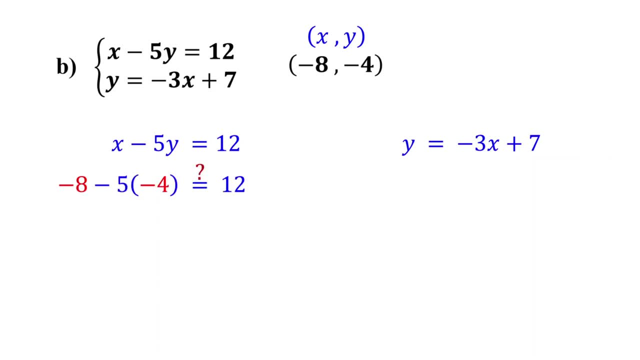 Starting with the first equation, plug in negative 8 for x and negative 4 for y. Negative 5 times negative 4 equals 20.. Negative 8 plus 20 is 12, and indeed 12 is equal to 12.. So the ordered pair satisfies the first equation. 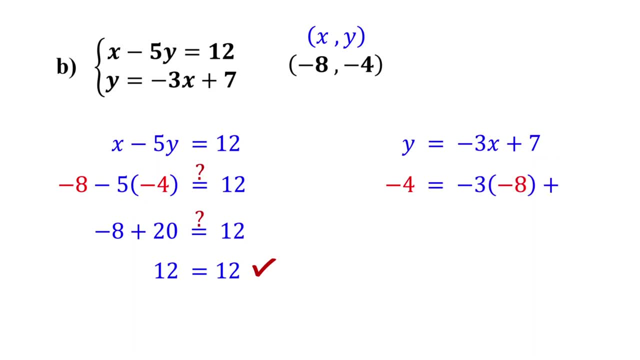 Let's see now whether it works for the second equation. Replace x with negative 8 and y with negative 4.. Negative 3 times negative 8 equals 24, and 24 plus 7 is 31.. But negative 4 is not equal to 31,, so it does not satisfy the second equation. 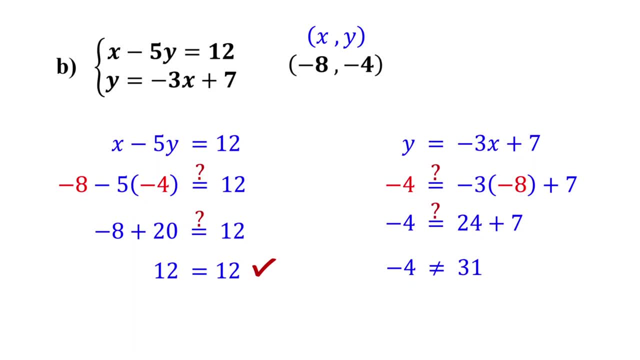 Remember that for an ordered pair to be a solution to the system, it must satisfy both equations. Since the ordered pair- negative 8 comma, negative 4, does not satisfy the second equation, it is not a solution to this system of equations. Now it's your turn to give it a try. 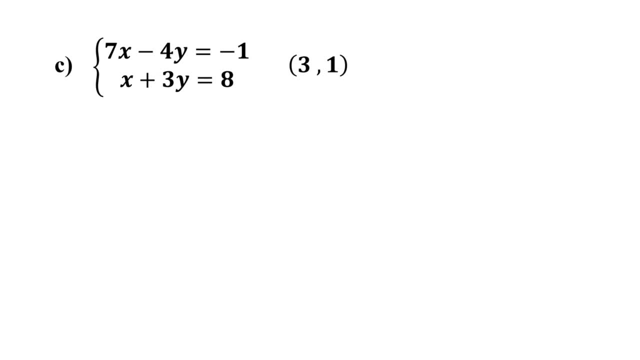 Is the ordered pair 3, comma 1 a solution to this system of equations? Feel free to pause the video and work on it. The x value is 3 and the y value is 1.. Plug in 3 for x and 1 for y. 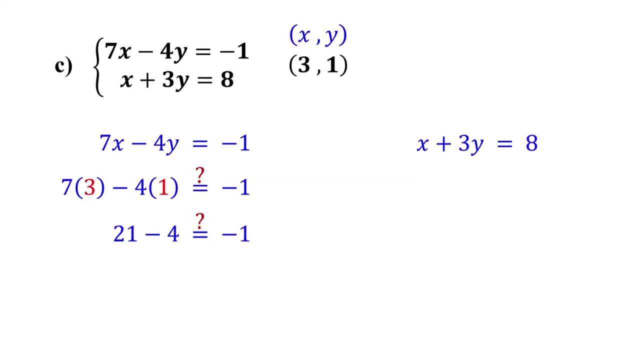 7 times 3 equals 21, and 4 times 1 equals 4.. 21 minus 4 equals 17.. However, 17 is not equal to negative 1, so the ordered pair does not satisfy the first equation. At this point there is no need to check for the second equation, since it already fails to satisfy the first equation.